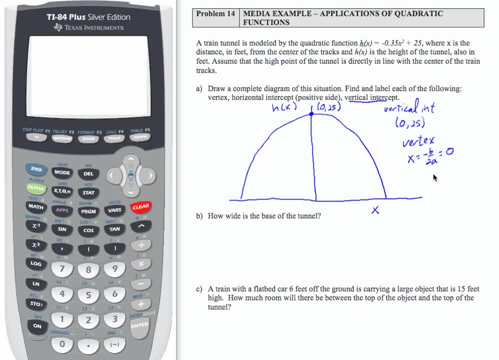 situation. So this is going to be when the input is 0, the output is 25.. So I know the vertex is 0.25.. So the vertical intercept and the vertex are the same thing. Now to find the horizontal intercept. 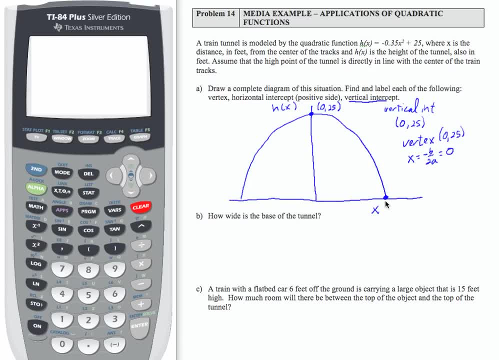 which is this point. right here I'm going to have to use my calculator. So let's go to Y equals and enter the function: negative 0.35X squared 0.35X plus 25.. So that's going to be my quadratic function. If I look at my window, I'm going to 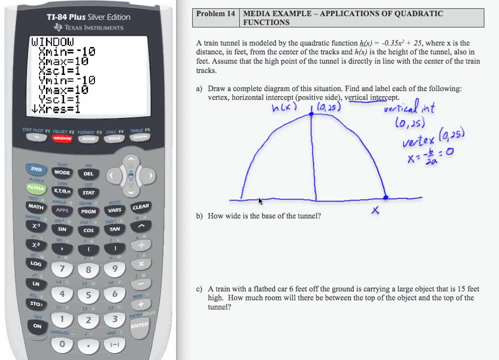 leave negative 10 to 10 because we want to see if we can show this shape. But my Y min, I'm going to make that 0.. And my oops, that was my X scale. I don't want my scale to be 0.35X squared, So I'm going to. 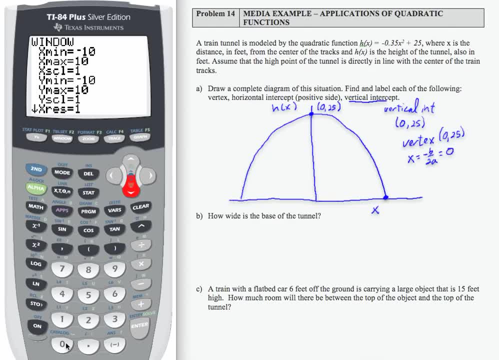 I want my Y min to be 0.. Here we go. And then my Y max I want to be, oh, let's say, 30, just so we can get it above this point right here. Now let's graph And let's see what happened here. Ah, I forgot my. 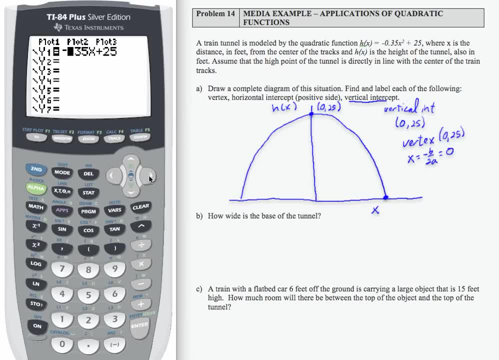 square on the X. That's why that looked like a linear function. So let's go over here and say insert, So second, insert a square. There we go Now let's graph. That looks a lot better Now if I. 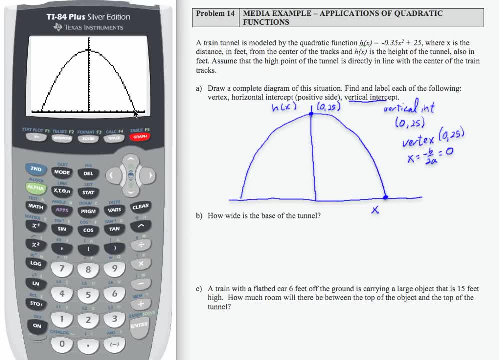 want to find this ordered pair right here. I need to intersect the quadratic function with an output of 0.. So I'm going to need to go back in and put 0 for Y2 and then go to second calc, number 5.. And I'm going to move that cursor just a little bit over to the right, Then hit enter. 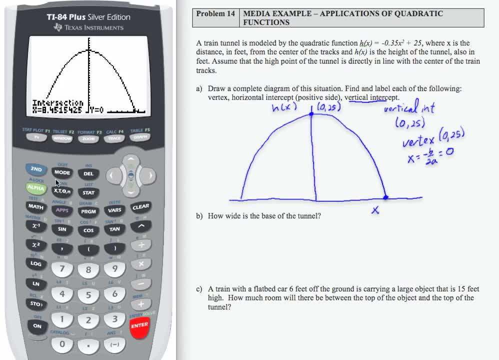 three times. So that gives us an intersection of 8.45.. And it doesn't tell us how many decimals, So I'm going to say just two decimals: 8.45 comma 0.. So this gives us a really, really good image of our situation. To find the width: how wide is the base of the? 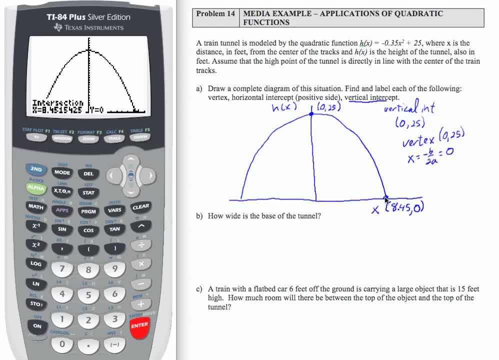 tunnel. Well, the tunnel goes from here to here, So all I'm going to do is take 2 times 8.45, which is 16.9 feet. So the tunnel is 16.9 feet wide. A train with a flatbed car is 6 feet. 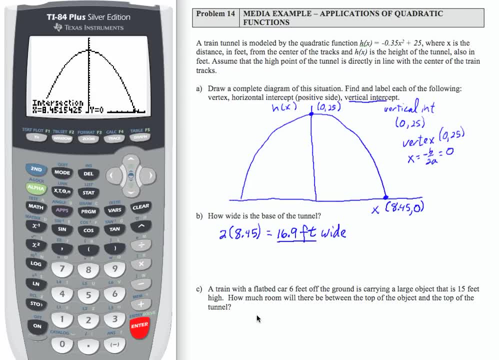 off the ground. It's carrying a large object that's 15 feet high. So that's 6 plus 15 equals 21 feet. Well, how high is my tunnel? That's going to be 25.. So 25 minus 21,. I'm going to. 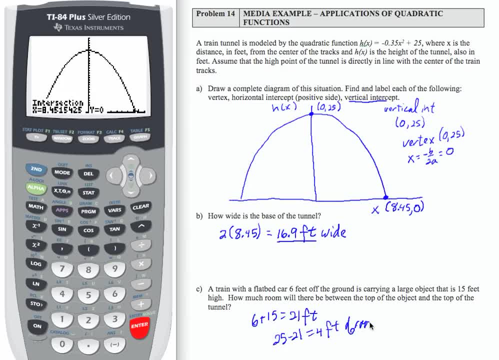 have 4 feet of room between the train and the cargo and the top of the tunnel. 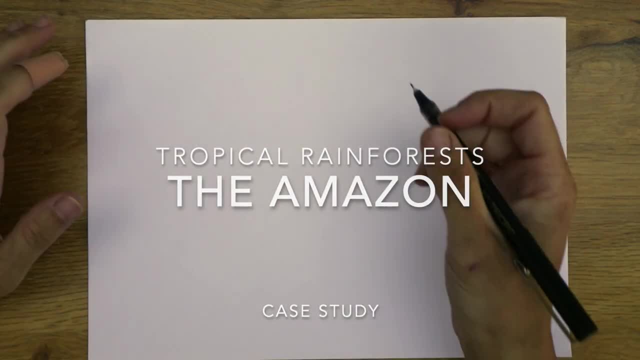 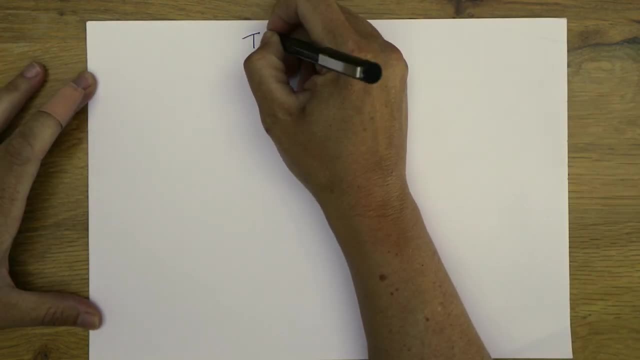 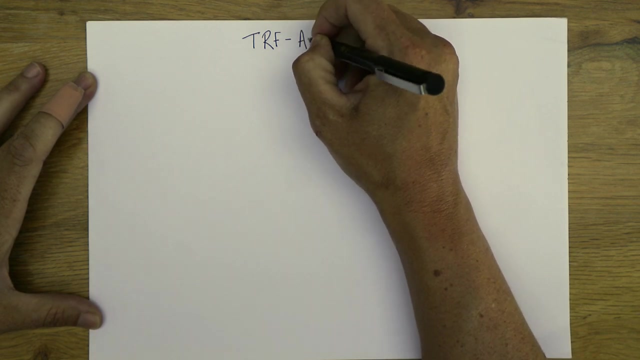 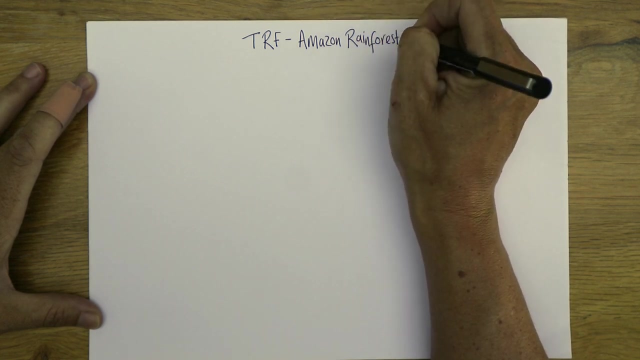 Hey folks. so I want to take you through one of our biggest case studies, and that is tropical rainforests, or TRF, and we're going to have a look at specifically the Amazon rainforest. Now, I know there's others that we can study, but for this 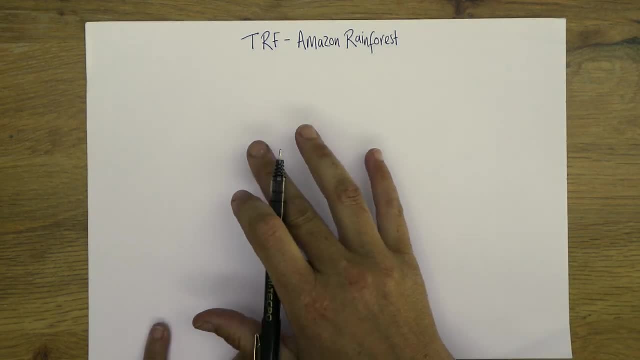 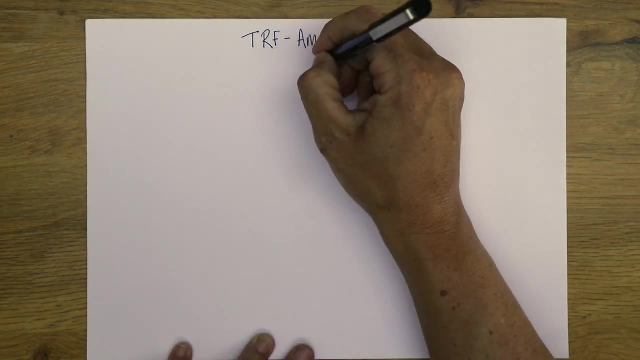 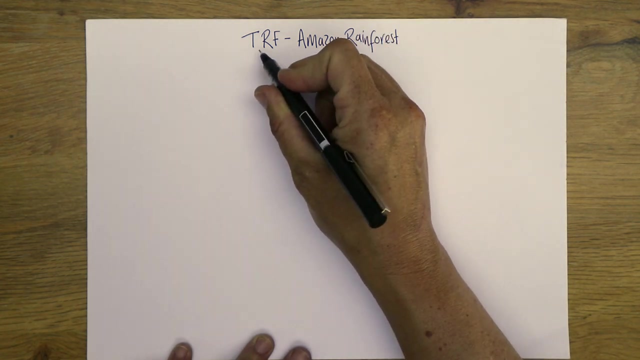 one. I'm going to try and simplify it as much as I can, but this one is gonna hopefully cover everything you need to know really in one infographic. Okay, so the first thing we just need to look at very, very quickly, if we imagine this, is the Earth, this little circle, and the reason they're called tropical rainforests. so you have the equator that wraps its way around the planet, and then, either side of the equator, you've got the tropics, the Tropic of Cancer and the Tropic of Sulfur, of Capricorn, and it's between those two that we find tropical rainforests, and generally speaking, they have an average temperature of 27 degrees Celsius, and that's what we need. we need high temperature and we also need that daily rainfall which comes from and is linked to that temperature. if you're thinking about your global air circulation model, which you might be, it's the Hadley cell.